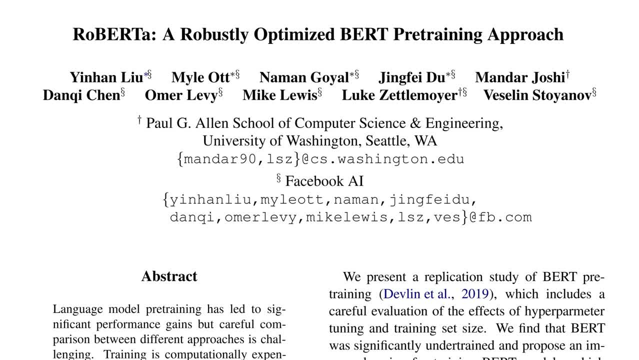 And this paper basically says: if you get the design choices right, then BERT- BERT is able to basically be on par or exceed all of these other methods so far. So they're basically exploring design choices in the pre-training and training of BERT. 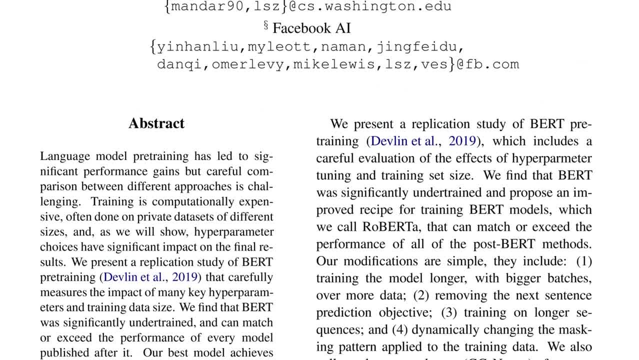 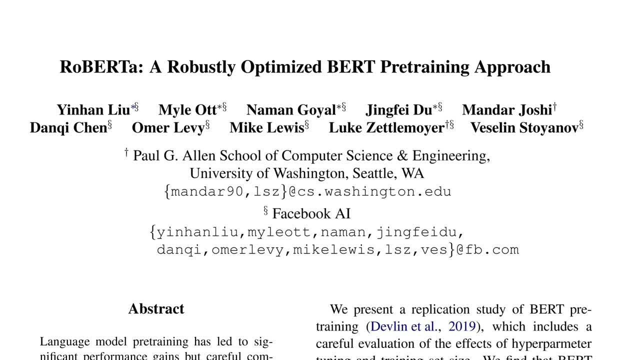 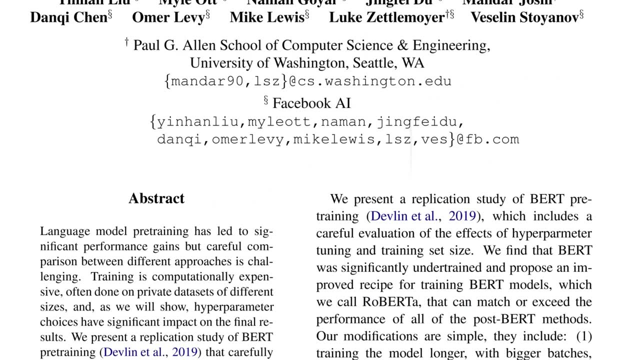 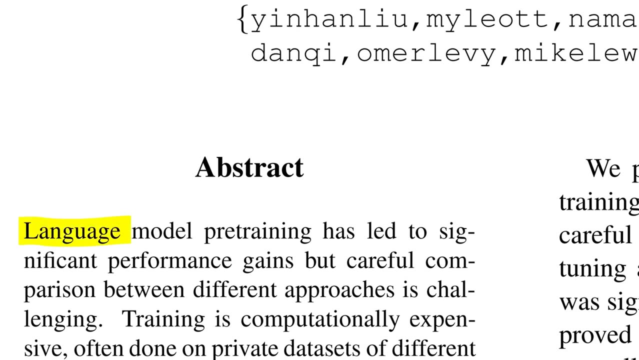 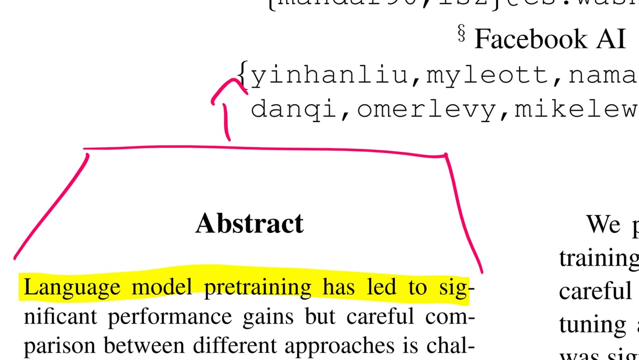 Alright. so if you don't know what BERT is, by the way, I have made a video about BERT. I've also made a video about transformers. In very quick terms, BERT is a language neuron. It's a neural network architecture that takes as input text such as this kind of thing you see here, text such as that- and it will kind of encode it out and it can do various things, for example, classify it into certain categories or kind of segment, it extract answers from questions and so on. 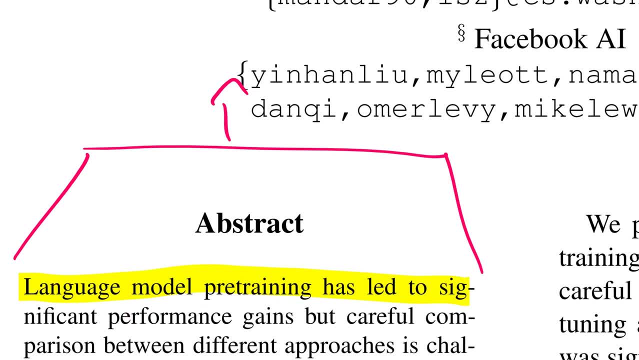 The whole thing is very simple. The whole thing is pre-trained with what's called a masked language model objective, where you don't need labels to train it. So in a masked language model objective, you basically mask out certain words during training and then you ask BERT to reconstruct these words from the surrounding information. 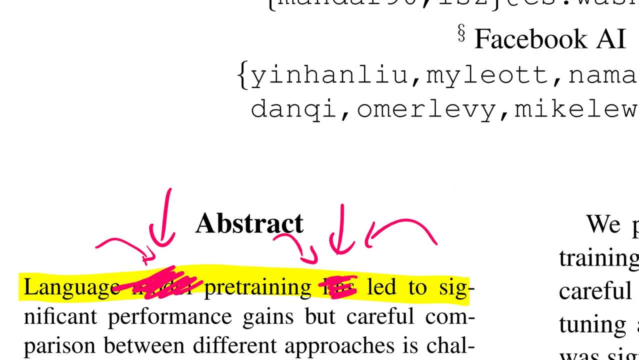 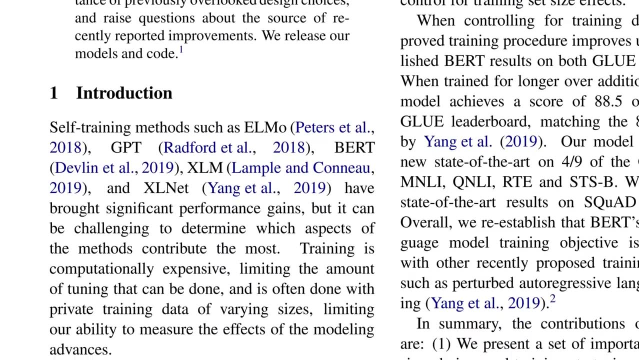 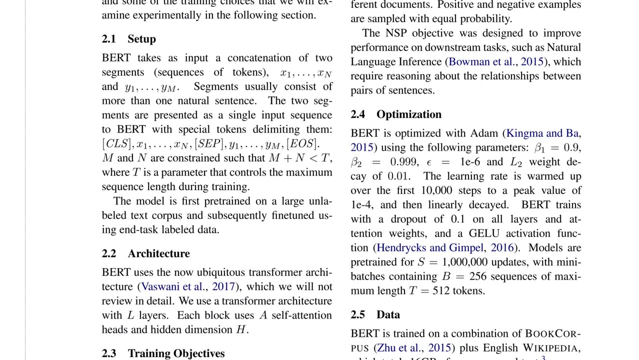 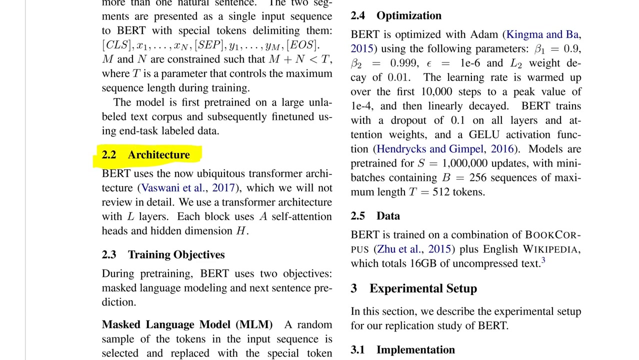 And that kind of has given some improvements in the original BERT paper. but subsequent papers have claimed that you can improve even more by using different pre-training objectives and so on, such as XL NET. but here these researchers basically explore different things. so they use a regular BERT architecture. that's what they describe here. so they use both the BERT base, the 12-layer, as well as the 24-layer BERT that has originally been described. 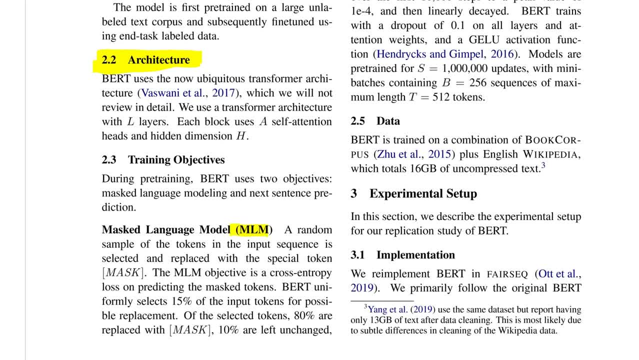 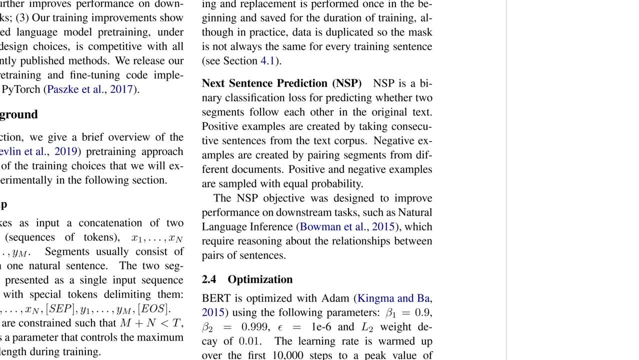 They use masked language modeling as a pre-training objective and they explore the necessity of this next sentence: prediction loss. that has been part of BERT. So, along with the masked sentence modeling, BERT has also had an objective where, if you input a piece of 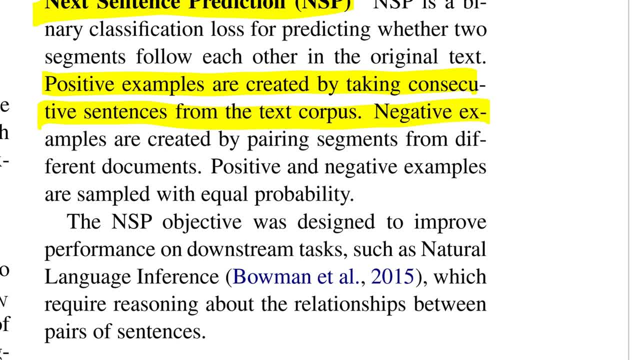 actually, you input two pieces of text, two sentences, such as this: these are two sentences and BERT has to decide if the second sentence follows the first sentence in the corpus or, in 50% of the cases, the second sentence is sampled from a different document. 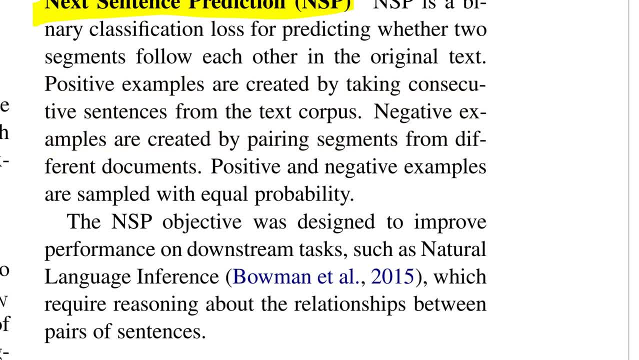 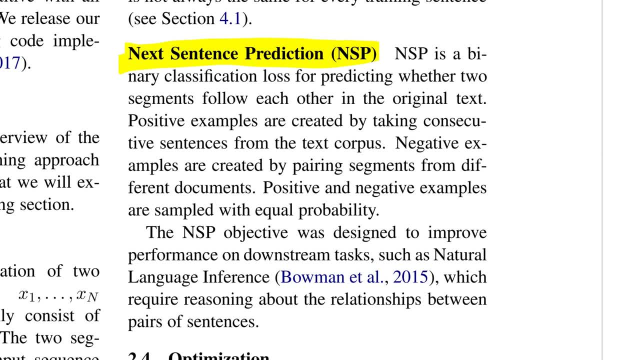 This kind of is So. the original paper argued this is necessary to incorporate long-distance relationships between text. Yeah, here, the NSP objective was designed to improve performance on downstream tasks such as natural language inference, And this paper kind of explores the necessity of that loss. 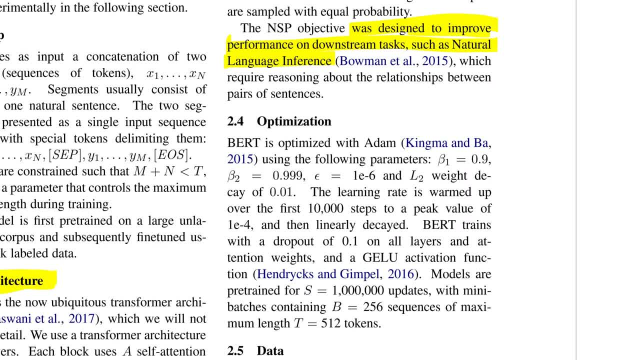 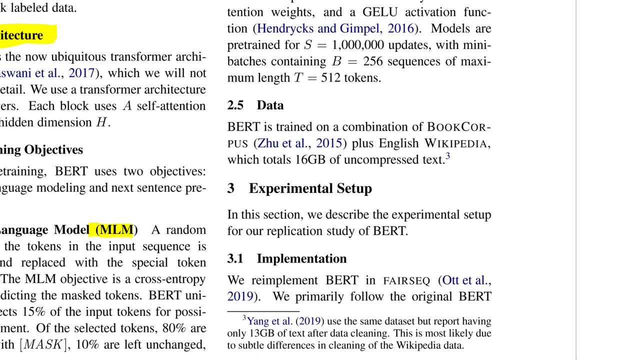 In terms of optimization. there is, of course, kind of a pre-training scheme and then a training scheme using Adam, here with certain parameters, And also this paper explores the use of these parameters. Lastly, you have data and, of course, these models. sometimes they're trained on different data. 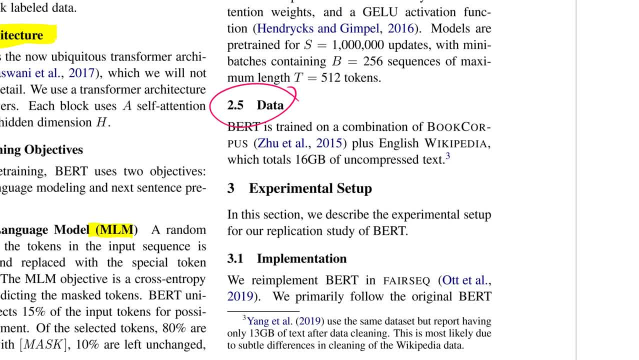 and that's why comparing them makes it a bit harder to compare them, because the pre-training is done on differently sized and differently structured data. This paper also tries to investigate the influence of the training data and especially what happens if we keep the training data constant. 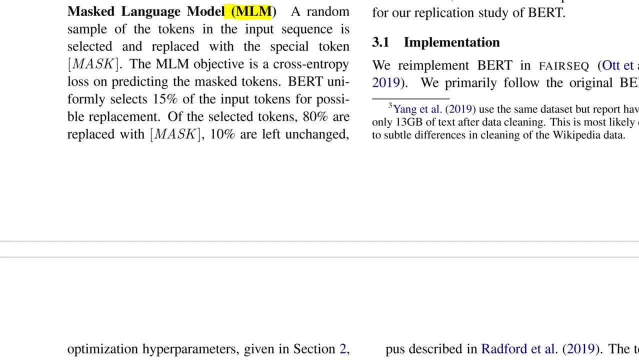 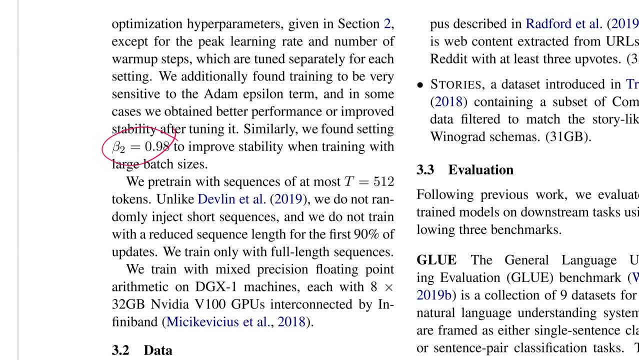 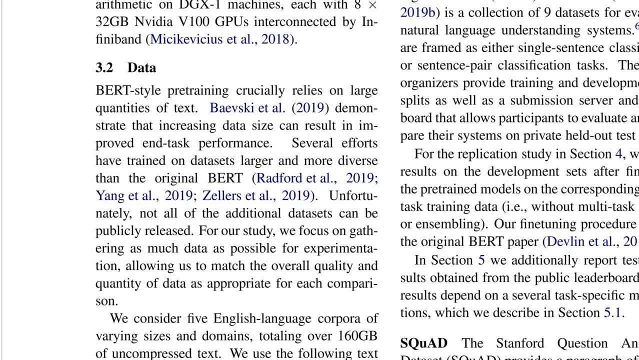 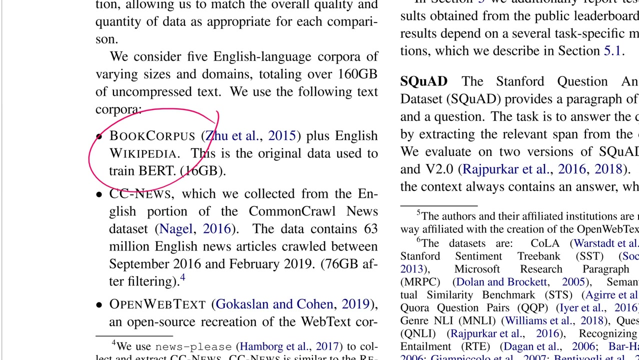 So Alright, so they implement BERT, they re-implement BERT and then they fix some hyperparameters, Um, While they tune others, And first of all the data set. So they use different data sets. The original BERT has been trained on this BookCorpus and Wikipedia- English Wikipedia data set, which is 16 gigabytes large. 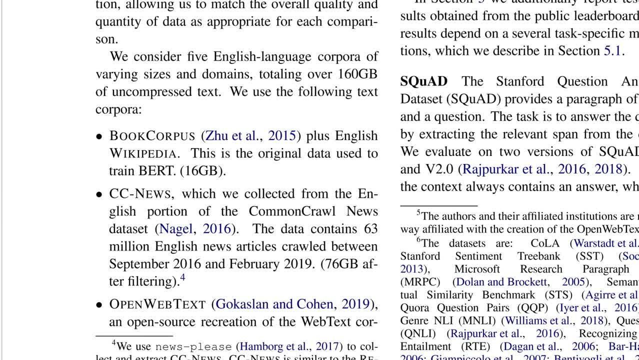 Now this paper here collects a- What's This? CC News data set, which is a subset of the Common Crawl News data set, which is all in. So the subset is the English portion and that's 76 gigabytes. 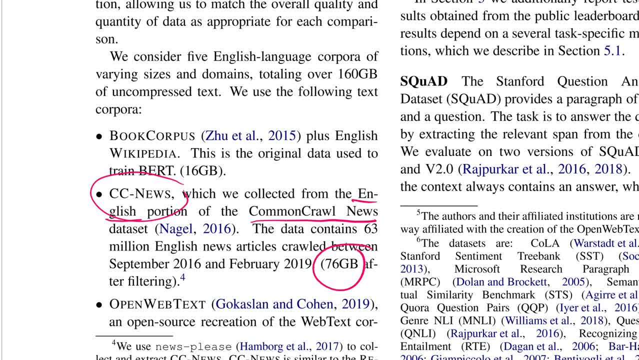 which is um on par with, for example, what GPT-2 used, I believe. So this is a very large training set and kind of comparing this original data to the large corpus, kind of what influence that is, should make very clear what the influence of more. 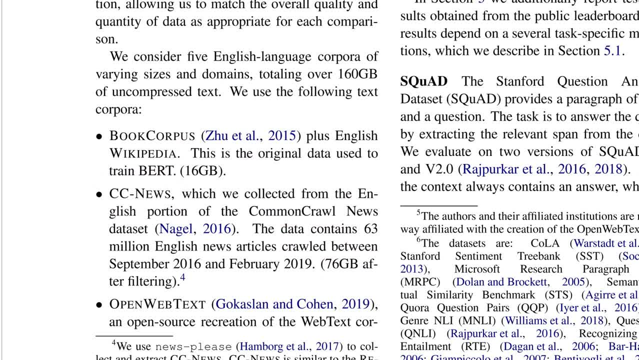 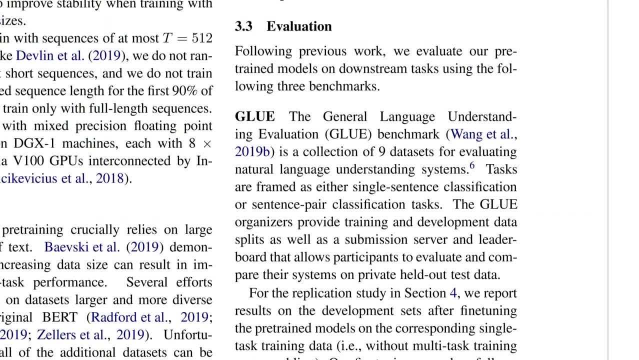 training, of more pre-training data is Now they also have a number of other uh corpora open web text as well as here. I believe there's one more stories. yes, So these are also uh pretty sizable. 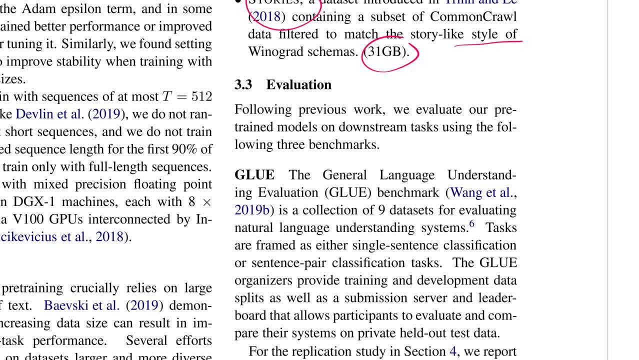 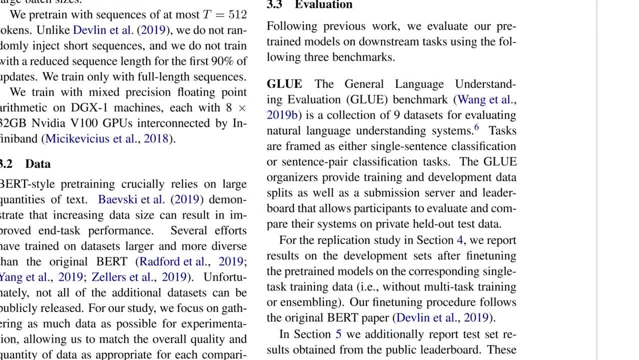 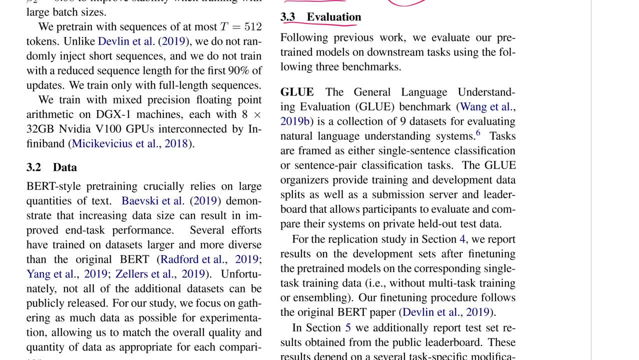 Uh, but these are like, yeah, these are like have very specific uh schemas to them. Um, then the evaluation here happens on several different kind of downstream tasks. so the idea is, you first you pre-train this BERT model on with the 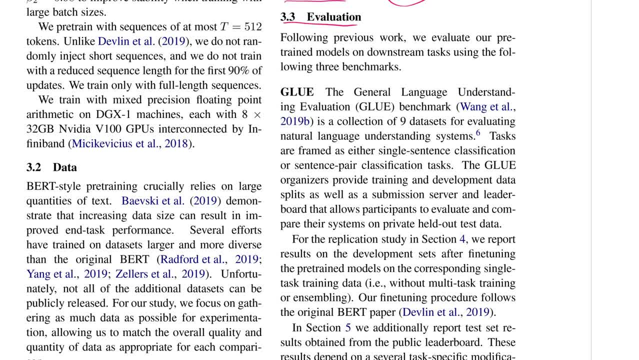 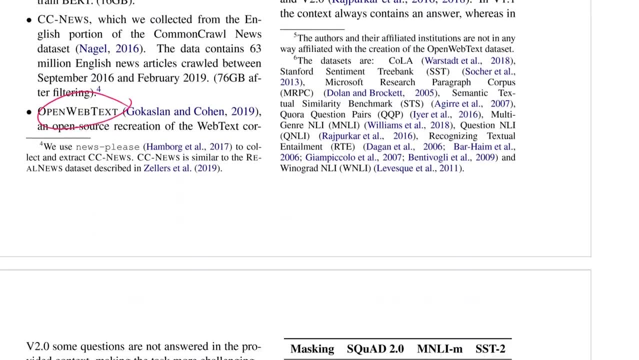 masked language, modeling and so on. and then, uh, you have this glue task, which is actually a collection of nine tasks, and, um, you have some, some other tasks, such as squad, which is a question answering task, and uh, here, 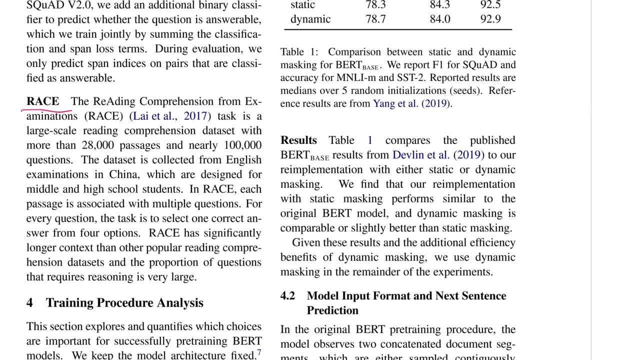 race. I don't even. I don't know what that is in particular, but suffice to say these are kind of downstream NLP tasks. The paper isn't about these downstream tasks, but it is just a way to measure how well your pre-training worked. 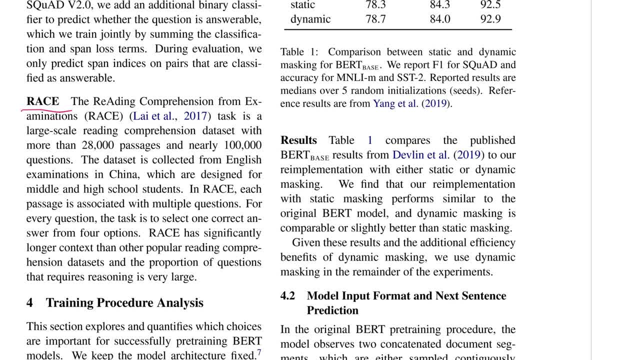 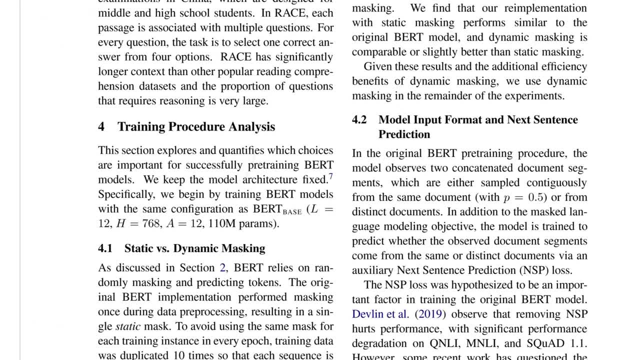 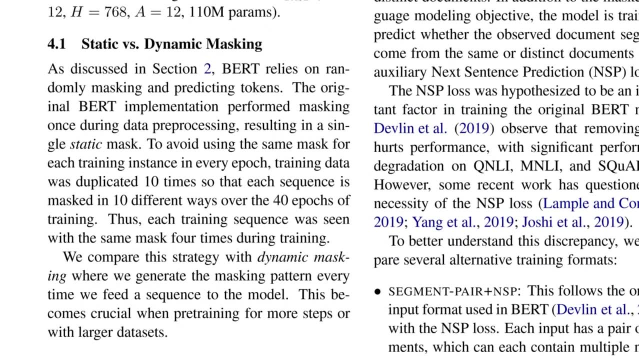 if then you can fine-tune on such a task and you get a good performance? Um, but what the tasks are in particular isn't too important. Alright, so here we get into the meat of the paper. First they, they- decide on what they. 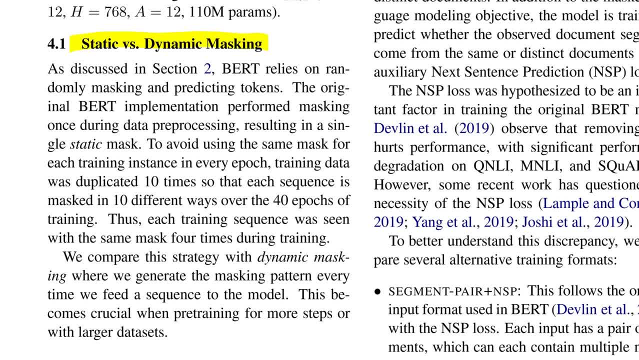 call static versus dynamic masking. So in the original BERT paper, whenever they do masked language modeling, they take a piece of text and they basically replicate it a bunch of times because they want to iterate through training data a bunch of times and then 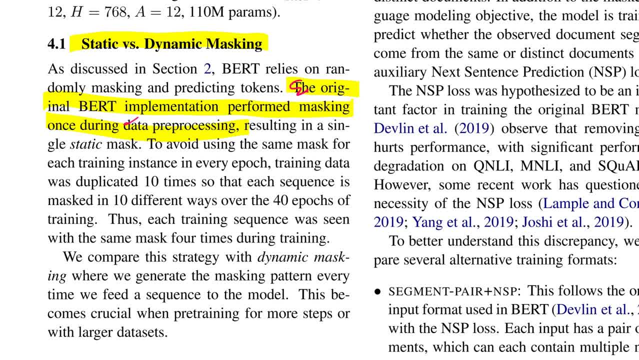 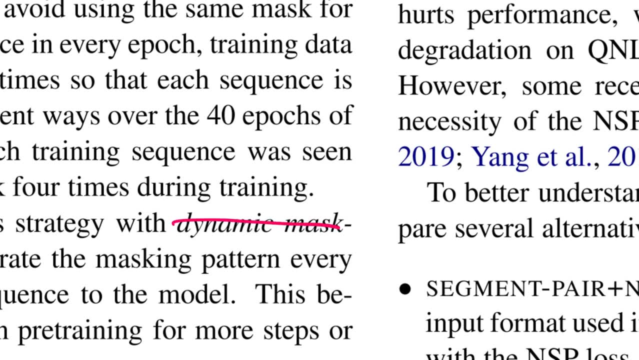 they in each iteration they mask out different tokens And um they compare the. they compare this to what's called dynamic masking. so this is static masking. Dynamic masking- sorry, dynamic masking would be where you um in each. 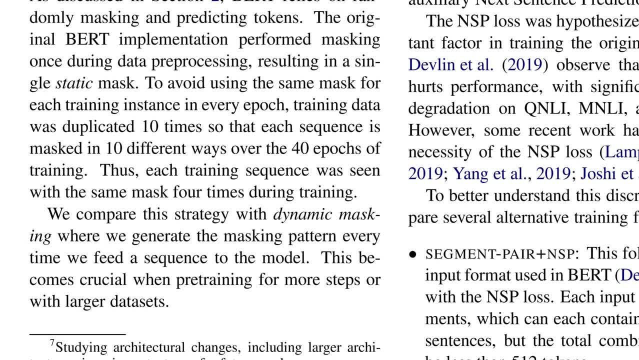 basically, on the fly, generate your mask. You don't pre-compute it and save it. you, on the fly, generate it. This allows you to go through kind of more or less of the data as you want and when you encounter the same sample twice. 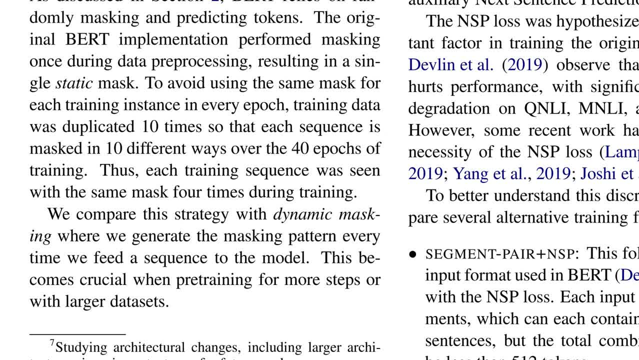 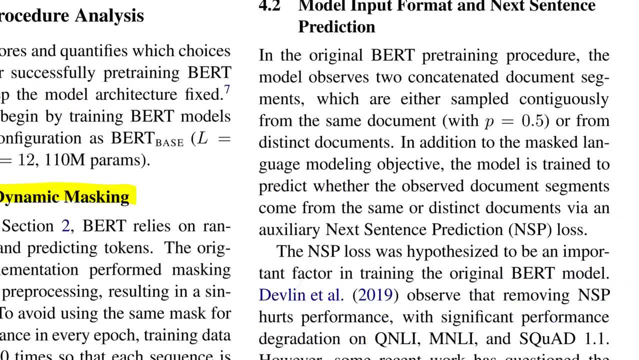 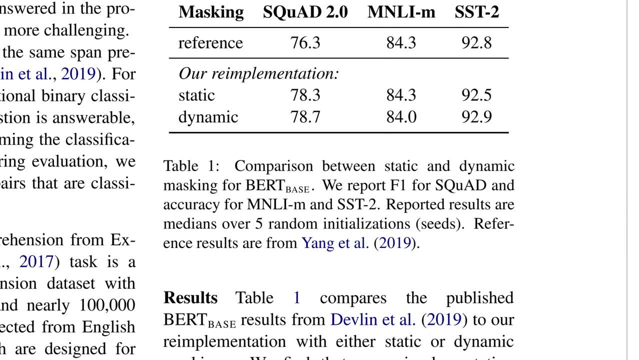 even though you replicate it in the original BERT model, you could still encounter it twice. if you train for longer than the number of replications, then you basically see the exact same mask again and the dynamic masking is actually much more useful. It's much more ad hoc. 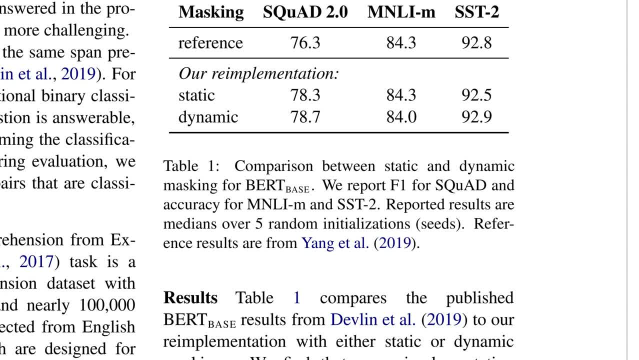 Each time you see a sample, you generate the mask on the fly. So they compare this here and they see that there is a marginal improvement. so here higher is better: Marginal improvement in two tasks and a less marginal decrease in performance in one task. So they 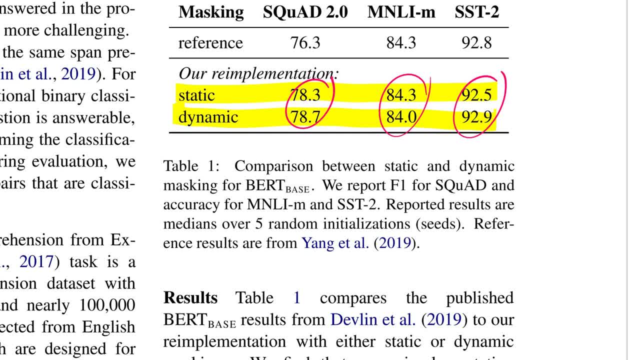 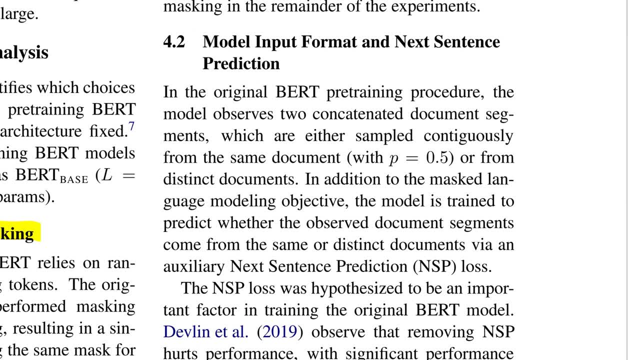 decide that this dynamic masking is of use. Second thing they investigate is the kind of input format and this next sentence prediction. So, as I already said, the original BERT training objective always gets two sentences next to each other and has to decide if the 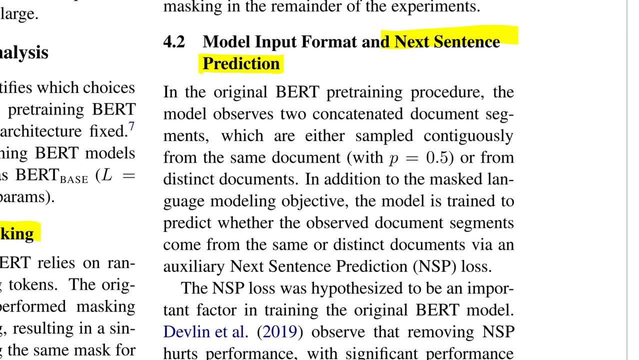 second one follows from the first one. Actually it doesn't. It observes two concatenated document segments which are either sampled contiguously from the same document or from distinct documents, And this is half and half. So, in addition to the masked language modeling, the model is 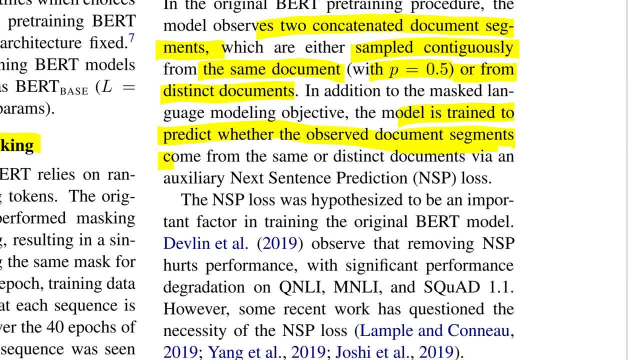 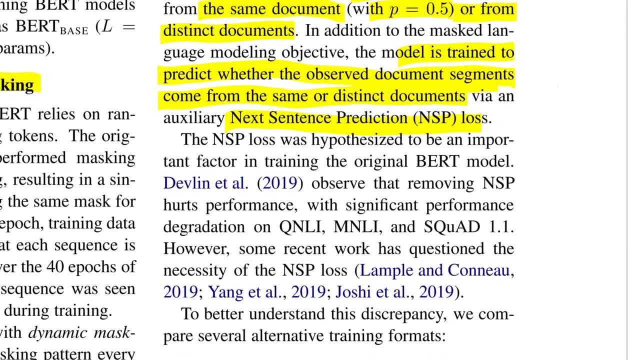 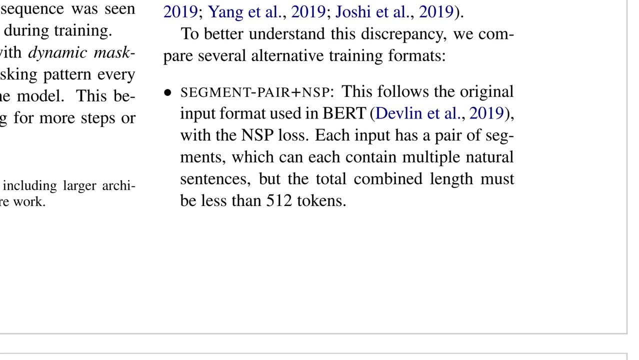 trained to predict whether the observed document segments come from the same or distinct document via an auxiliary next sentence, prediction loss, And they investigate different ways of including or excluding this loss. So first is what they define here. If it's plus NSP, that means that this particular thing. 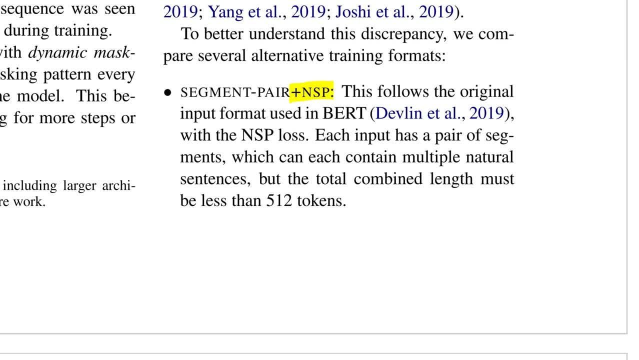 includes the next sentence or next segment prediction loss. So they have segment pair plus NSP, which means that each input has a pair of segments And these segments. now the distinction between a segment and a sentence is important. Where the sentence is really a natural sentence, a segment can. 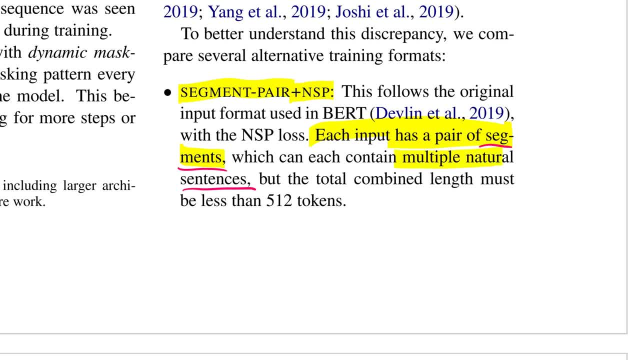 actually be multiple natural sentences, which is what the original BERT does. So as long as the combined length is less than 512 tokens, there can also be multiple sentences, but there's clearly two segments and you have to decide if they follow. 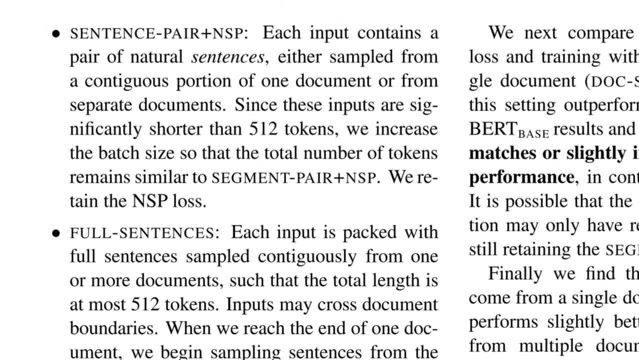 after each other or not. The second thing they try is the same thing. so the next segment prediction. but now it's just two sentences, It's just natural sentences, So it must be one sentence, a period, and then the next sentence a. 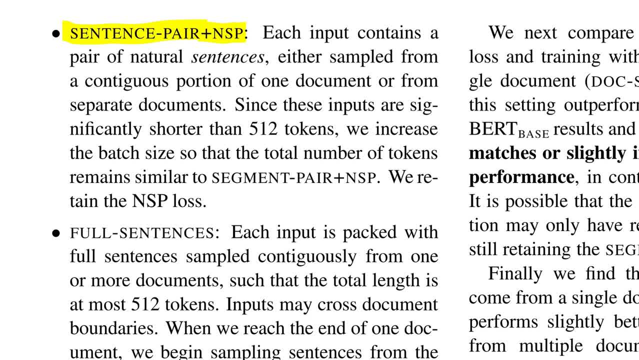 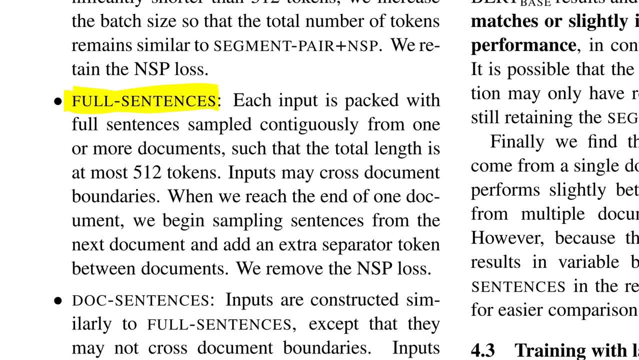 period and you have to distinguish these two, if they follow or not. Then they investigate full sentences, which is, they leave away this next segment, prediction loss, and they simply fill up the 512 tokens with text from the corpus. So each input is packed. 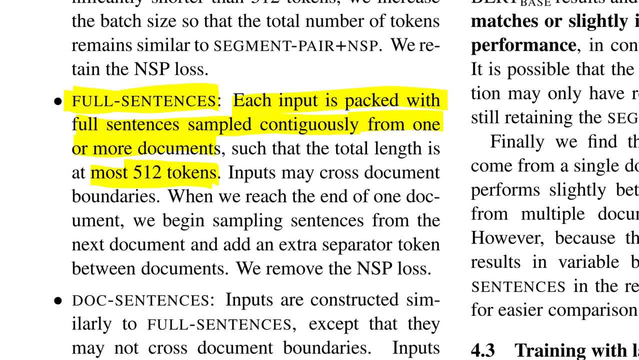 with full sentences sampled continuously from one or more documents, And the one or more document means if you sample text, you put all of this in the thing and you are at the end of a document. you simply continue with the next one and go on until. 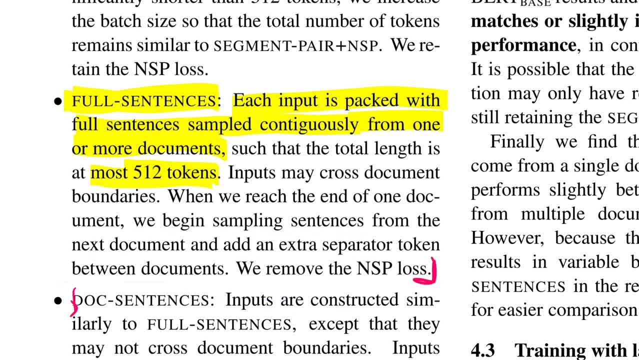 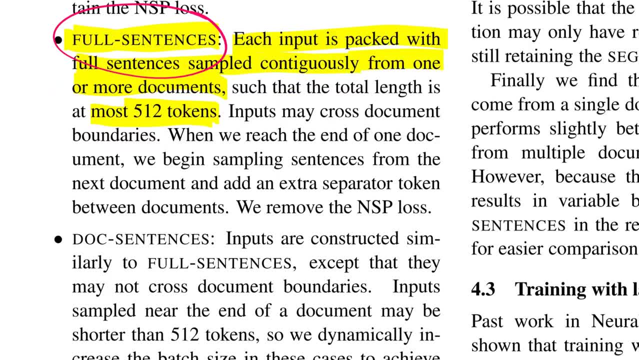 you have the 512 tokens. So you basically fill, fill, fill until you have 512 tokens, and that's this variant here. And then in the last variant you do the same thing. this is called doc sentences, but you basically: 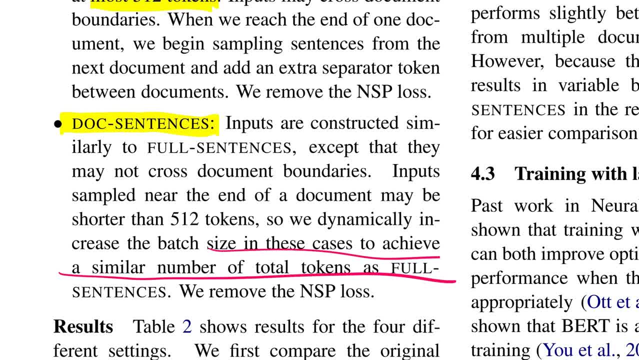 stop at the end. So you put all of this in your state and if you're here you stop. And then you have to be content by simply padding the rest of the 512 tokens or something like this, so you don't have as much. 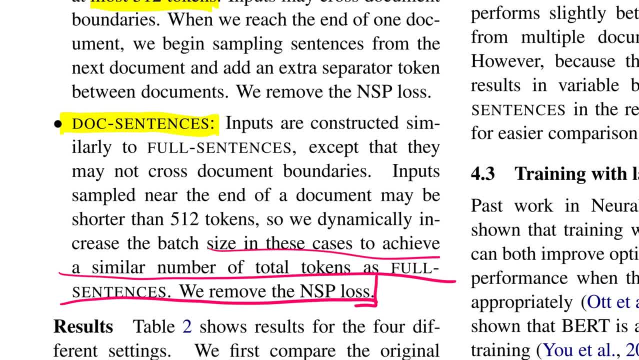 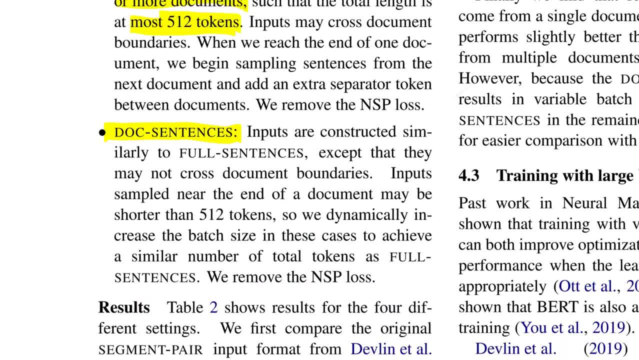 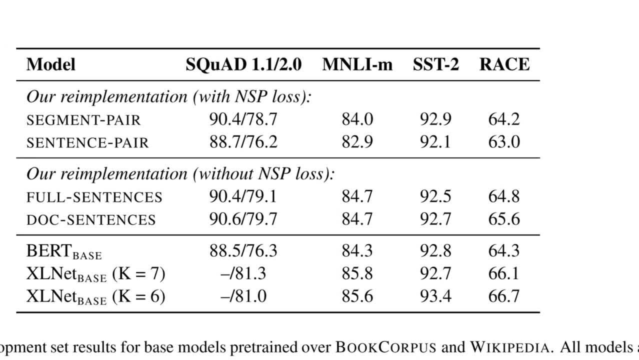 data, But the all the text that you have in one sample is actually contiguous text from the same document. So they pit these four things against each other. this is this table here and, as you can see here the best thing is this doc sentences: 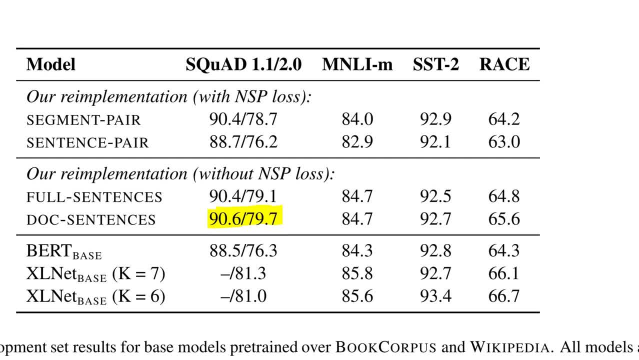 thing. so on these things followed by the full sentences encoding. So there's some ambiguities here, but in general you can kind of rank them as best, second best and then here third best and fourth best, And they conclude that this next segment or next, 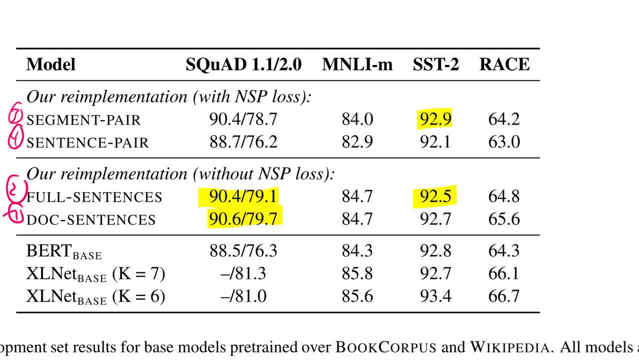 sentence: prediction loss here is more hurtful than helpful in the ways we see here. And they say, even though this is most effective in their case, they'd rather go with this one because it's easier to implement. you get more data. 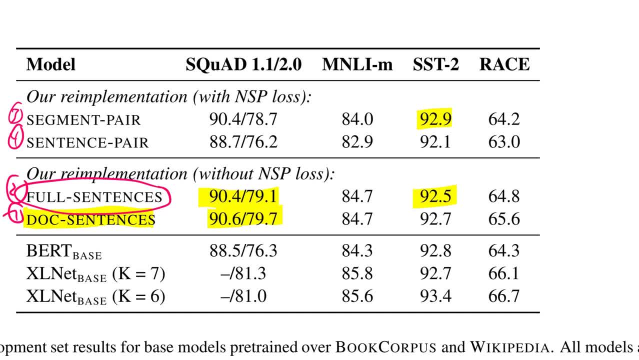 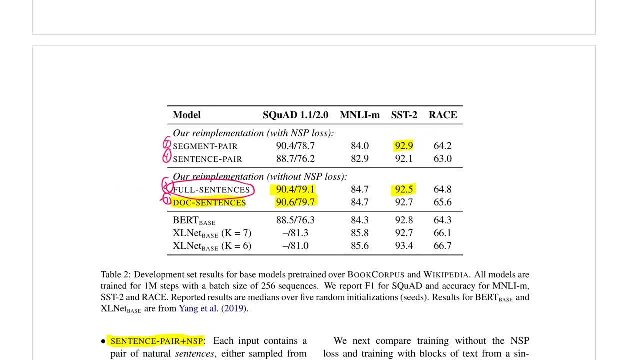 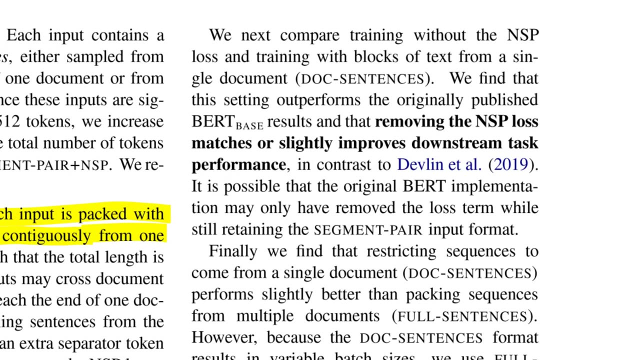 through the model in the same time and the performance decrease isn't that much. But it's pretty interesting to see that this next segment, next sentence, prediction isn't super, super helpful in actuality Here. so removing the NSP loss matches or slightly improves the 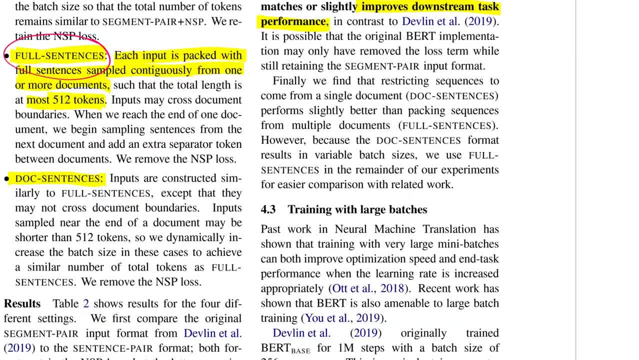 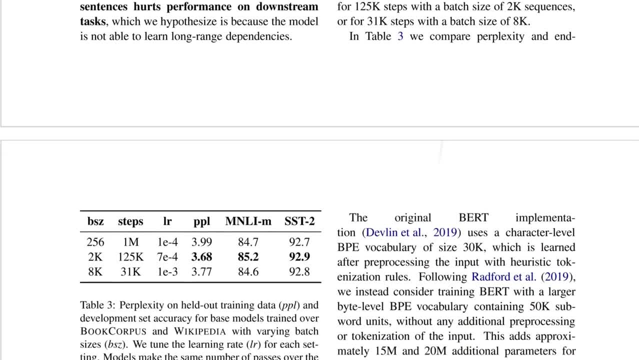 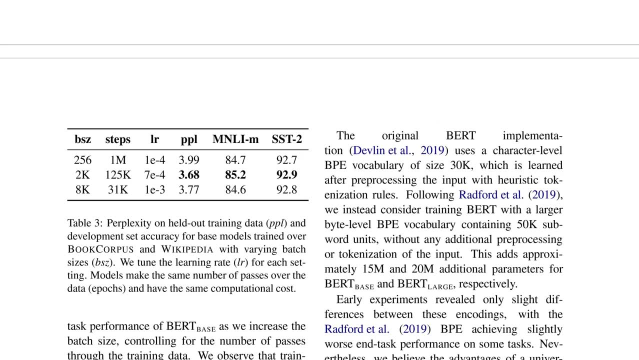 downstream task performance. This is yeah, in contrast to what the original BERT authors found. but you have to keep in mind this is also on has a bunch of other changes in. Then, next thing, they investigate batch size. So batch size. 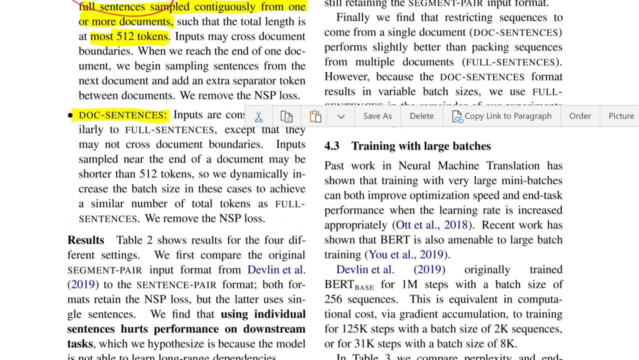 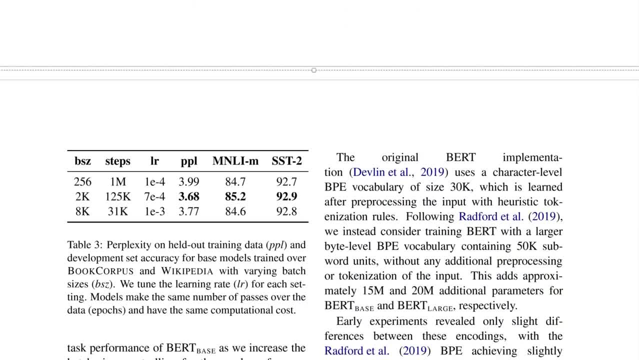 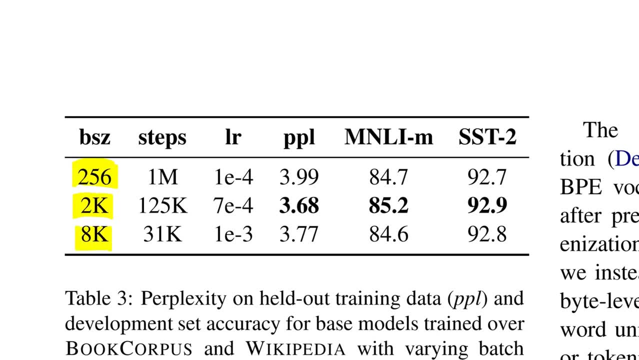 sorry, batch size pretty seems to be pretty interesting for these large models in that they love large batch sizes And they actually explore batch size sizes: 512 here as the smallest one, and they go up to 8000.. So this they do this. 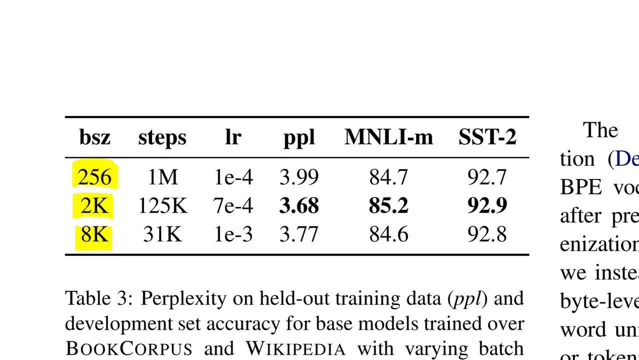 actually in a data parallel way, where they have many, many machines with many GPUs and they parallelize the data and then they accumulate the gradient of all of these different samples, and so they can go up to a batch size of about 8k. 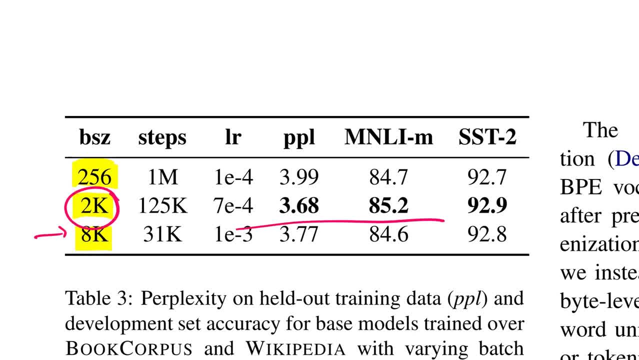 And they find generally that the 2000 batch size here, as you can see, helps to improve the. so perplexity: lower is better and if the other number is higher is better helps to improve the performances. if you control, they control. 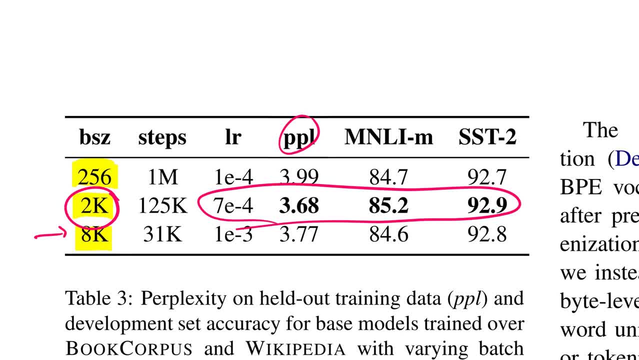 for data set size. so the number of times you go through the data set is the same. but if you go with a larger batch size, that seems to help up to a point. Here the 2000 seems to be the best they found, So again, 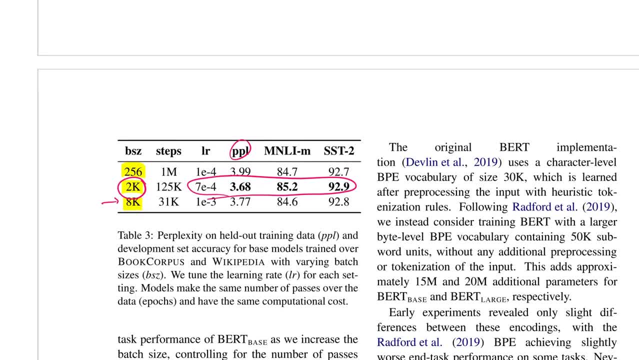 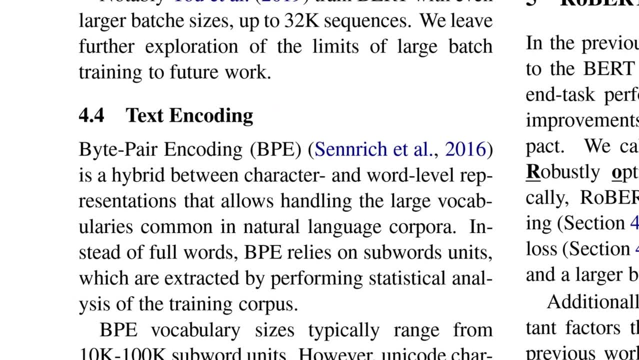 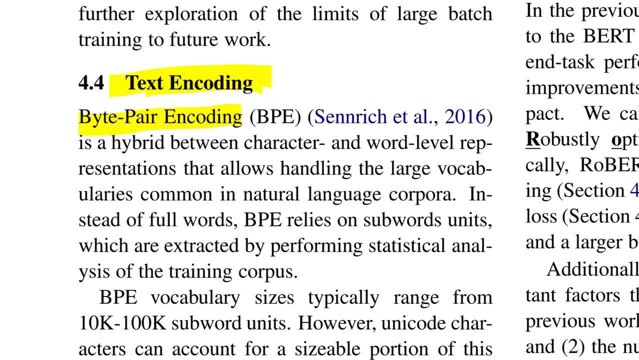 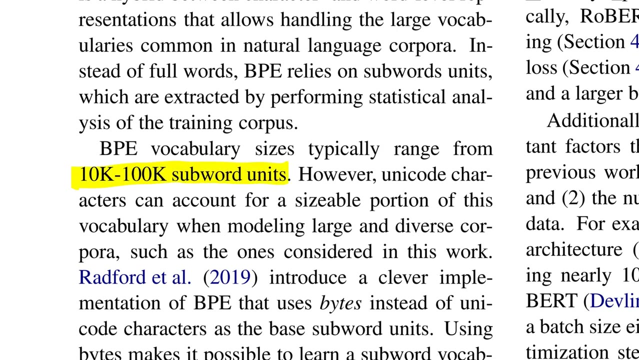 marginal improvement you can make by training with larger batch sizes. And then the last thing they've looked at is text encoding. So how do you encode text? And the pit here is basically between byte pair encoding or word piece encoding to decide how large your. 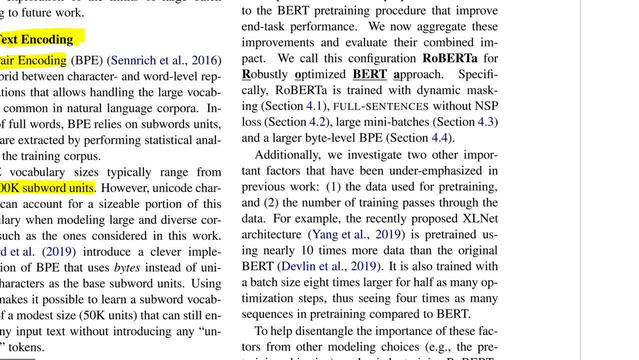 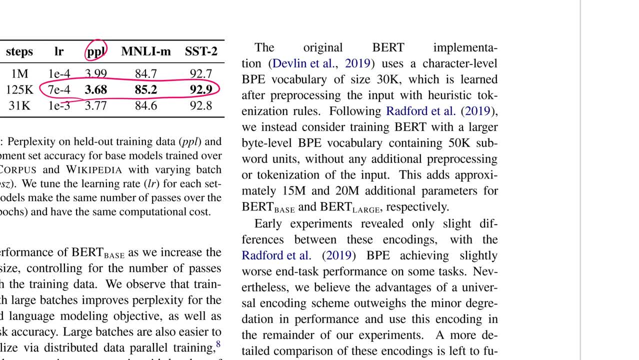 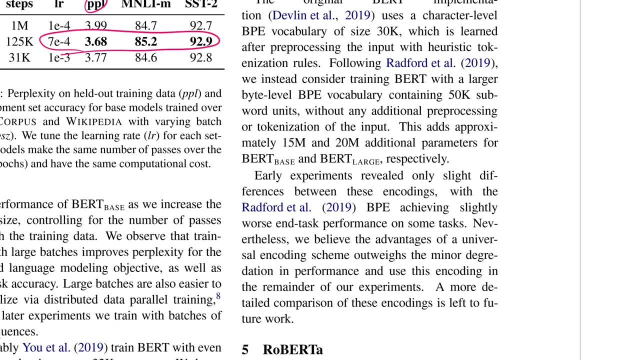 vocabulary is basically, And, as I understand it, they didn't find much of a difference between the different implementations of the text encoding, so they decide they go with. they decide to go with one. I don't even remember which one I think they decide to go with. 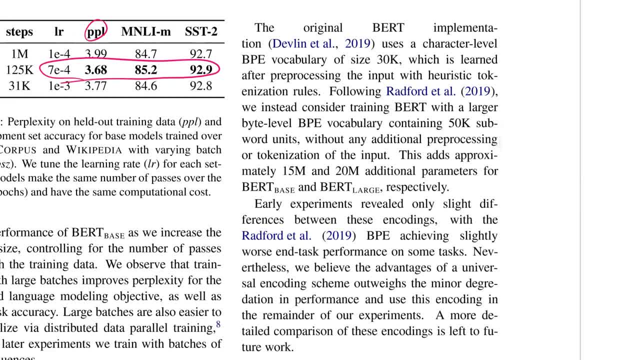 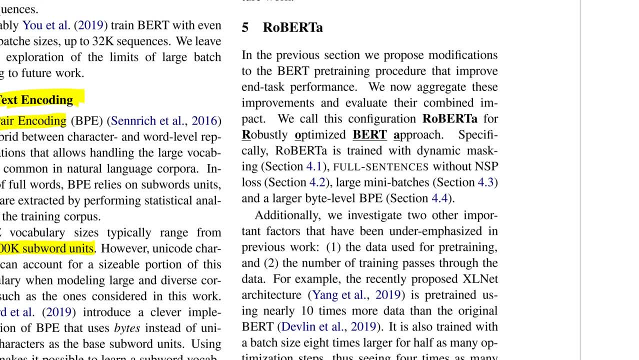 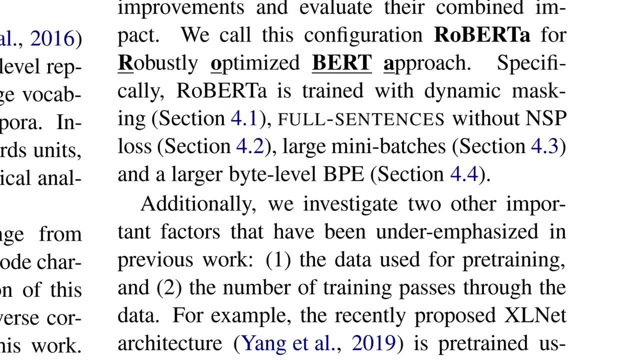 byte pair encoding instead of word pieces. Alright, so they combine all of this into ROBERTA, which is the robustly optimized BERT approach, and they say: ROBERTA is trained with dynamic masking. so what they showed? first full sentence without the next. 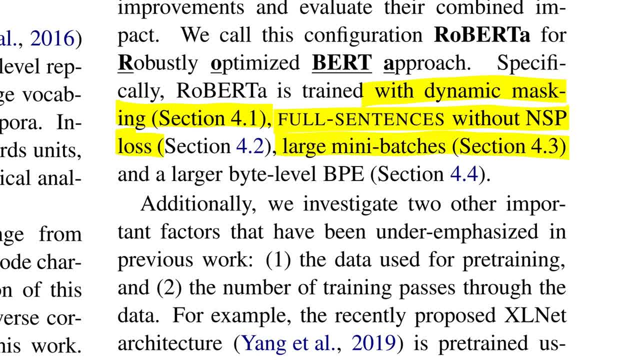 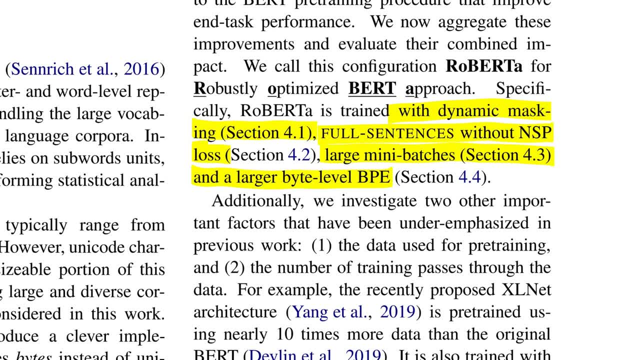 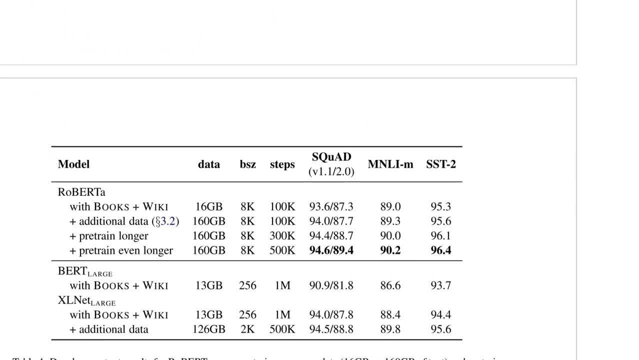 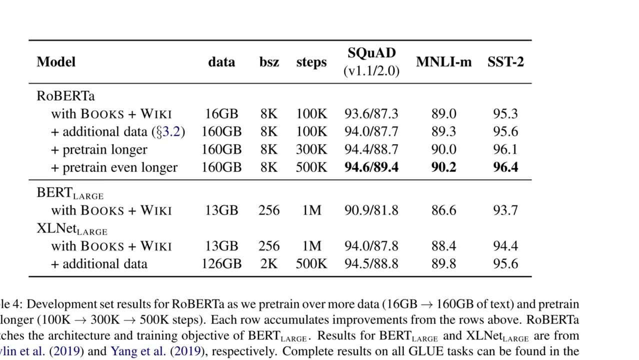 segment prediction loss, large mini batches, a larger byte level, byte pair encoding, as well as, of course, their collection of training data. And then here they also investigate how long to pre-train. So if you look at the original BERT models or the 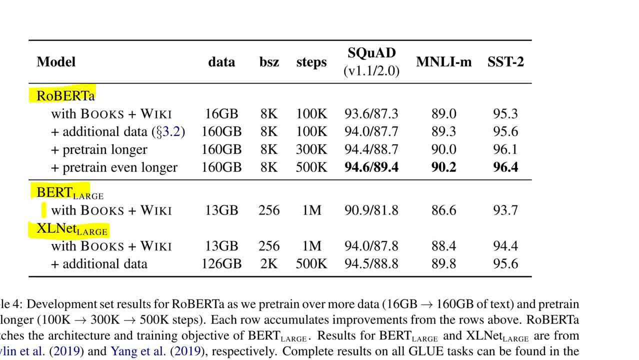 XLNet models and then compare it to ROBERTA. So ROBERTA, this is the original data And they already beat BERT, yet they do not yet beat XLNet with that. So if they add data, they get even better. 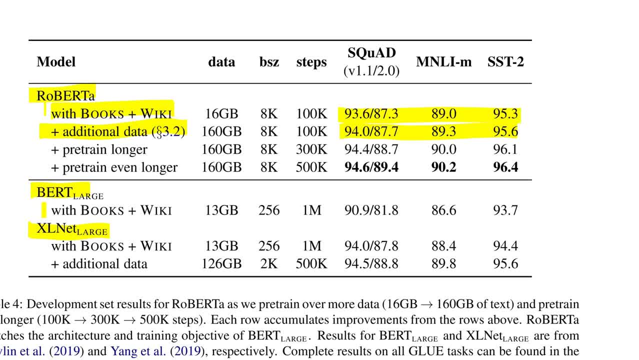 Actually on par mostly with XLNet. If they pre-train longer, they get even better, And if they pre-train even longer, right. so here's the number of steps. If your number of steps then match the number of steps that the 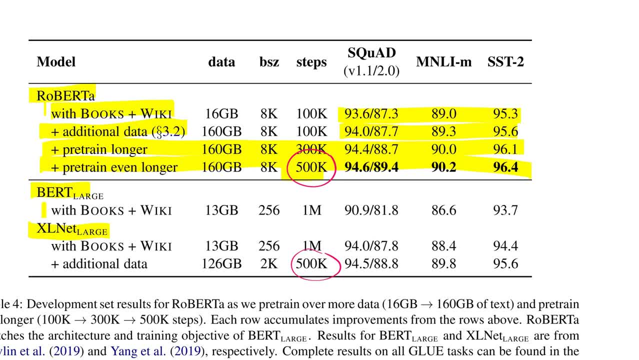 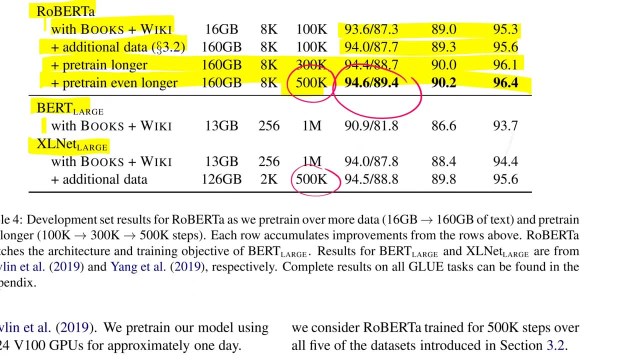 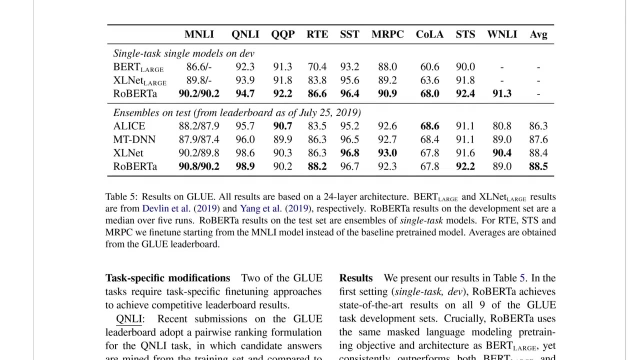 XLNet does. with the same additional data then, or with their additional data, then you outperform XLNet as well. So this is kind of just an overview of this. And they evaluate on other downstream tasks and they basically show that in most of them they can reach. 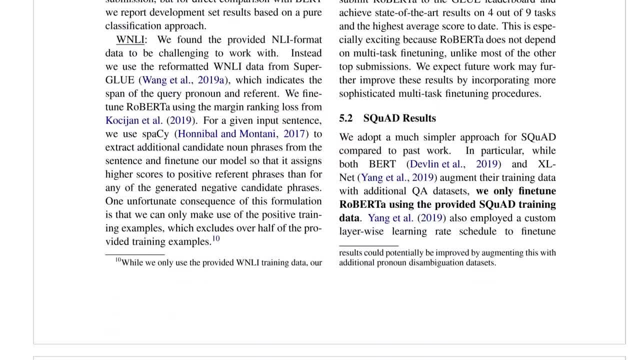 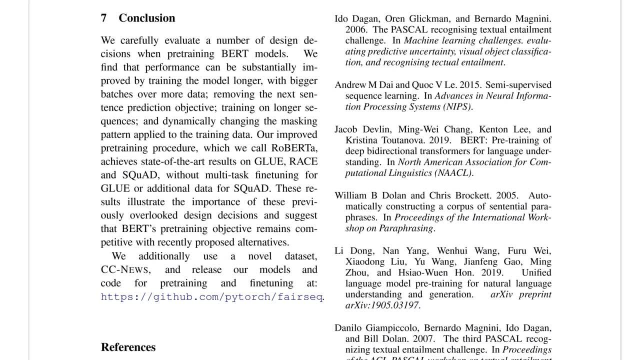 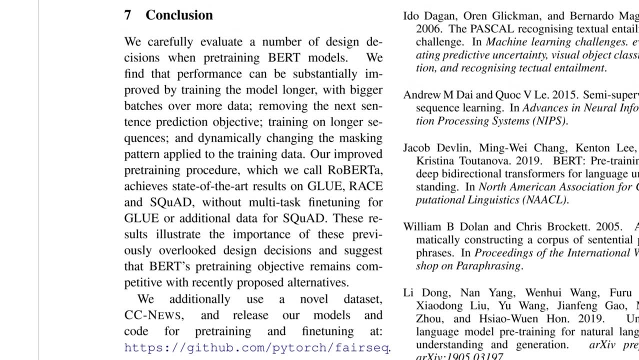 state-of-the-art performance or exceed it with their approach, And in conclusion, they basically say: well, this only shows that kind of the gains that these other models make, and the reasons why they make gains may be questionable If you simply pre-train, BERT. 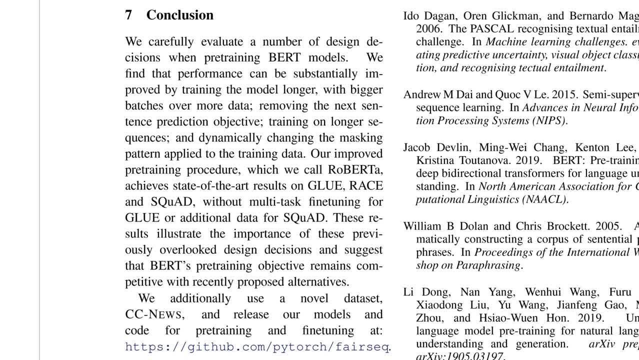 in a better way you can reach the same performances. So I think the end is not reached yet. Most of all, they publish their code, their data. I believe I have not looked into this, But definitely check out their repository where this is implemented. 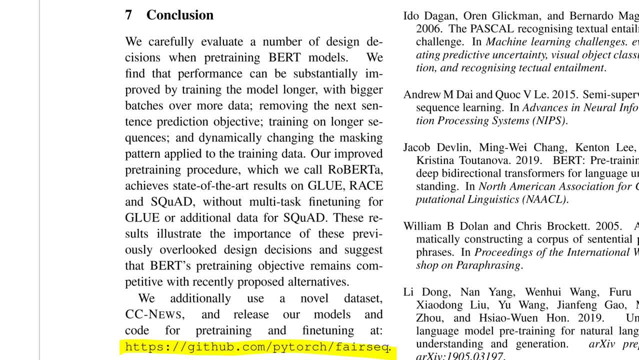 Seems pretty easy, seems pretty straightforward, And that was it for me. Bye-bye.